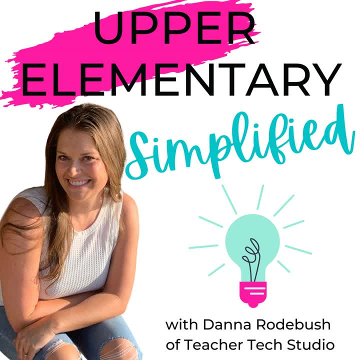 Are you ready? Let's simplify. When you think of guided math, what do you think of? Do you think only? Do you think only about small group instruction? Well, I am here to tell you that guided math is much more than just small group instruction. 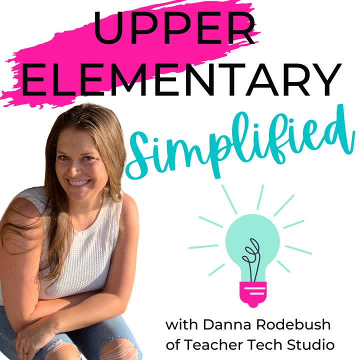 In fact, small group math instruction makes up only a portion of the type of learning that should be occurring in a guided math classroom. When I was writing my blog series all about guided math, I came up with my own scholarly definition of guided math. 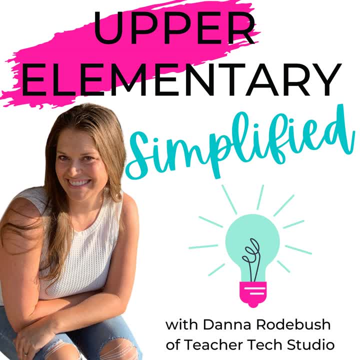 And I'm going to read that for you now. It says: Guided math is the careful planning and implementation of a systematic method of math instruction designed to foster a deep understanding of mathematical concepts using a variety of instructional techniques. Now, that is just a wordy way of saying guided math uses lots of different types of resources and teaching methods to help all students. 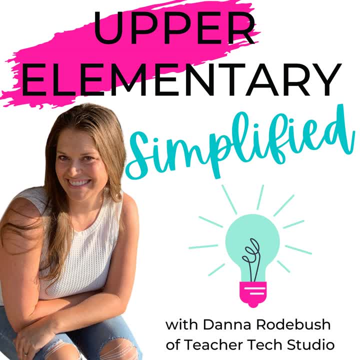 be successful in learning math skills. Put another way, guided math is a structured set of math instructional strategies that allow for targeted instruction, student engagement and a deep understanding of math concepts. This nine-part series of Upper Elementary Simplified is sponsored by the Ultimate Guide to Guided Math for Upper Elementary Teachers. This free guide includes: 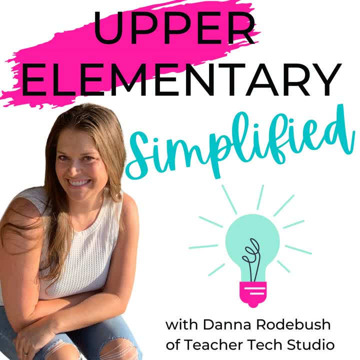 43 pages of practical and useful tips for you to learn about guided math, including how to implement this powerful instructional strategy in your upper elementary classroom. Download your copy of this free resource by heading to teachertechstudiocom forward slash guided math book. That link will be in the show notes So you may have searched for ideas about how to implement. 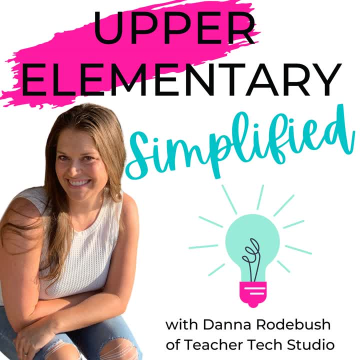 guided math in your classroom And come up with a list of instructional strategies and activities, with terms like differentiation, small groups and intervention thrown in. But what does all that mean for your upper elementary classroom? Today? I am going to briefly list the 13 components that I believe. 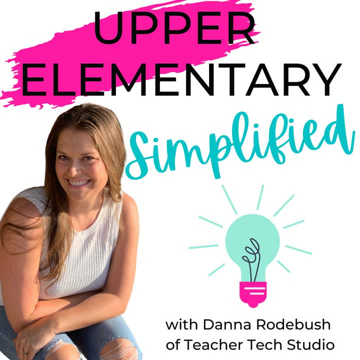 are essential to an effective guided math schedule. While 13 may sound like a lot, it all flows together smoothly and could really be parallel. So let's get started. I like to be very thorough in my explanations And then, over the course of the next several, 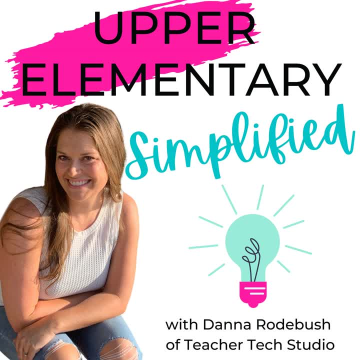 episodes during this nine-part series. I will be breaking down the components into further detail. The first component of guided math is whole class instruction with guided note-taking to introduce a new math skill. The second component is guided practice that immediately follows the introduction of the new skill, which is then quickly followed by the third component. 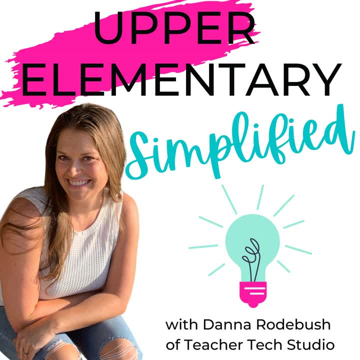 independent practice. Number four is a formative assessment to gauge the comprehension of your students during the whole group lesson and practice Component. number five is a mini review math lesson with more guided practice. The sixth component of guided math is an emphasis on vocabulary. 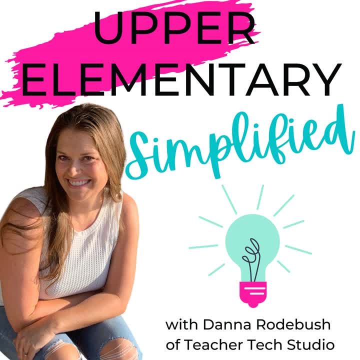 This is actually an often overlooked important piece of the guided math classroom, and it's the importance of vocabulary instruction and contextual use of math vocabulary. Upper elementary students should be regularly given the opportunity to use math-specific words in context, as they are mastering a new skill. Number seven is lesson warm-ups throughout the 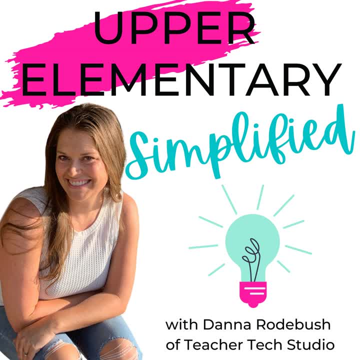 week to get students thinking. Number eight of guided math is small group instruction. The sixth component is manual ". The ninth component is to provide hands-on learning opportunities during small group and outside of small group. Number ten is formal and informal assessment. Number eleven is real. world application of the skill. Number twelve is viral text. Universal English learners and readers cannot agree with each other onねぇl-snovc's. began learning by there. normal Number twelve is a🤍 mensen more useful than usual. ar association. Number thirteen is lived upon. speech debate The number fourteen is textual instruction: value approximation. but you will be as one of us when it comes down to math, In bara, meeting with your master's classmates to share their story. German and evil as your homeroom for student. your master全部 deeto centers if you.